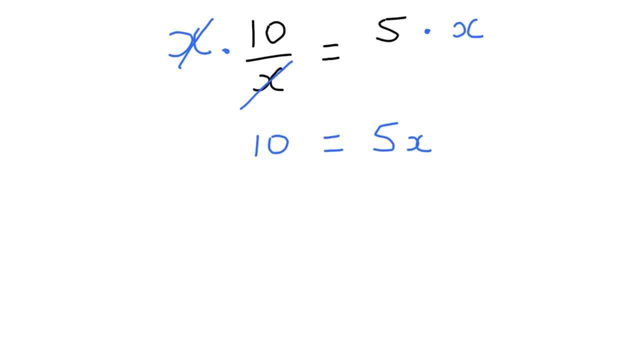 Now it becomes really easy to solve To get rid of the 5 on the right side. since it's 5 times x, I divide by 5. And I want to do the same thing on the other side And these two 5s cancel out. 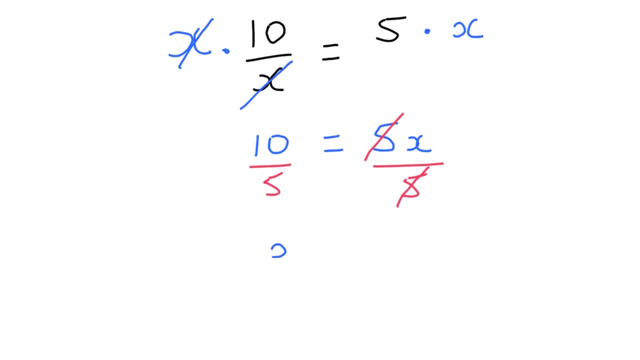 Now I have my x by itself On the right side. in math we usually switch it to the left side, So we get: x is equal to something, And 10 divided by 5 is 2.. Now what I want to point out is notice in my first step. 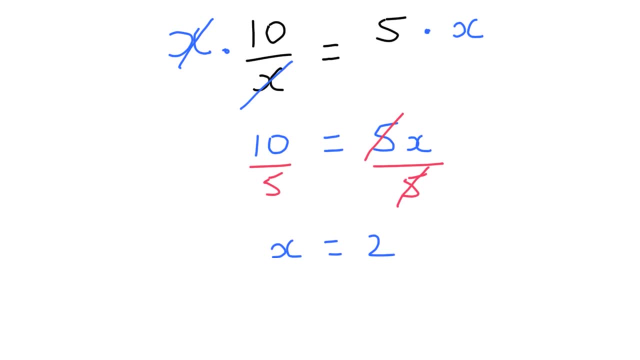 when I multiplied both sides by x. I'm writing the x up high, as if it's in a numerator, as if it was x over 1.. There's a lot of students who make the mistake of, when they multiply by x, they want to multiply it down. 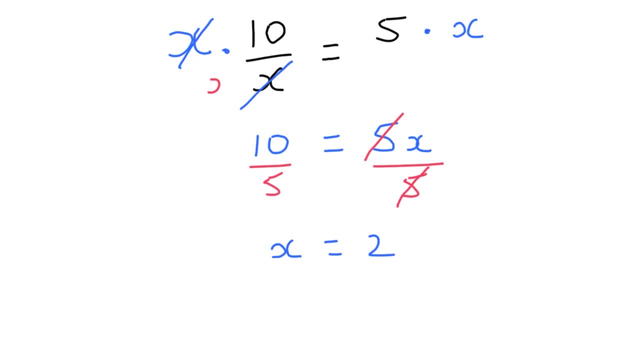 They want to write the numerator beside the x, But do not do that. I want you writing the variable up top, like this: So we have an x on top and we have an x on the bottom. 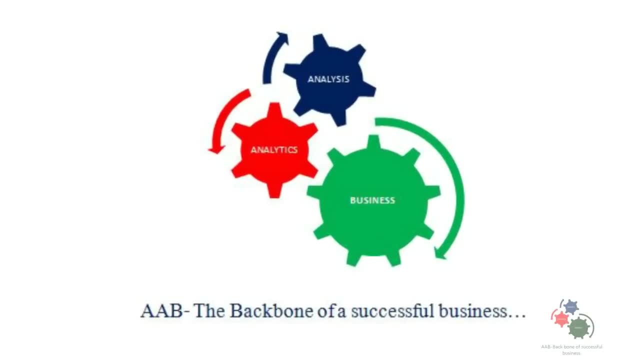 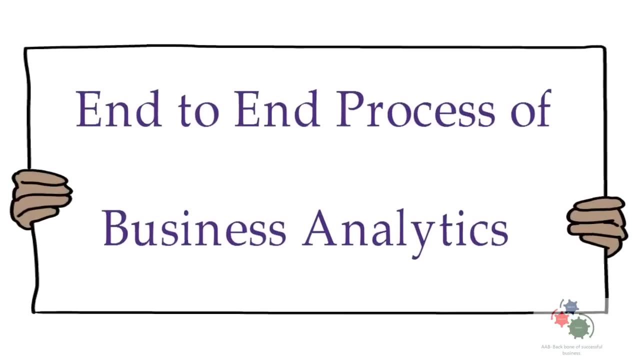 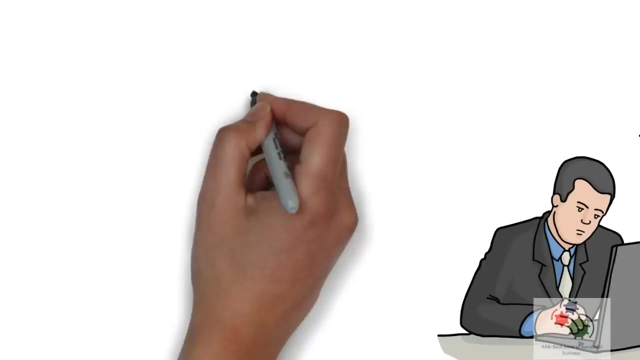 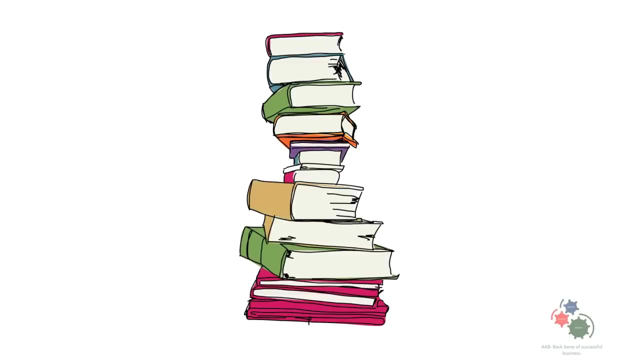 Hello friend, welcome to AAB Here. in this video I'll explain most used end-to-end process of business analytics. When I tried to learn business analytics, I had struggled a lot to get entire end-to-end process in one place. That is why, after reading lot of 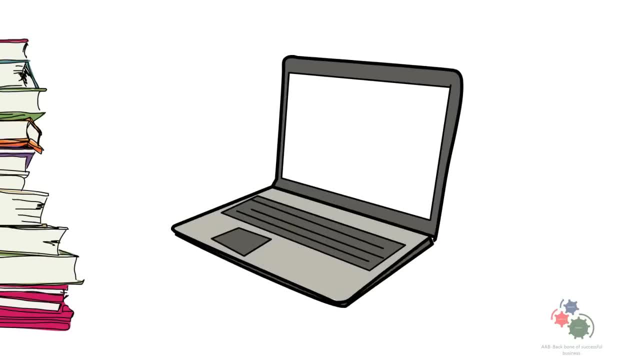 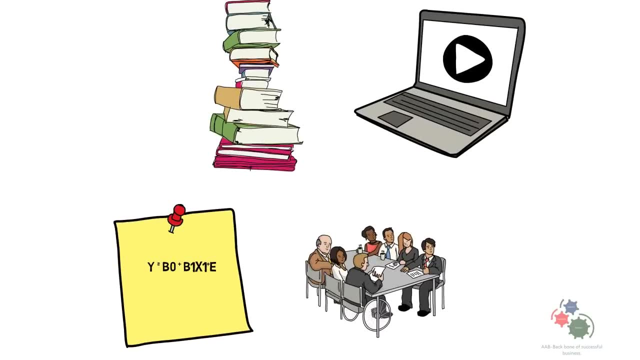 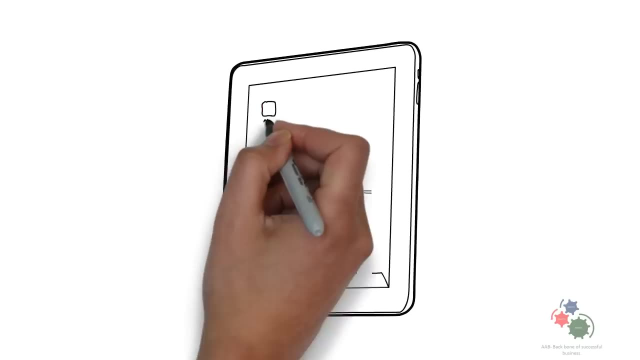 books, discussing with friends and colleagues, watching lot of videos, doing lot of research. I have come up with these videos for you, friends. I value your time and effort. That is why I'll try to give maximum content in this video. One video can solve your maximum problem. 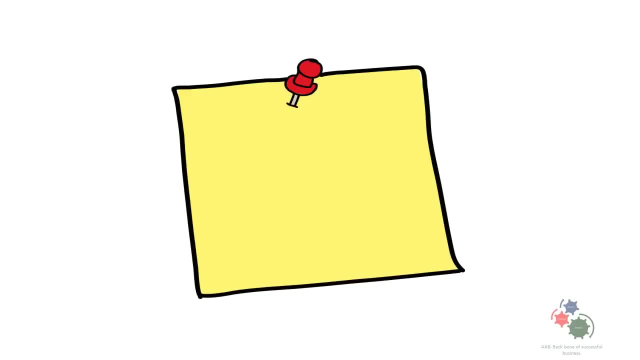 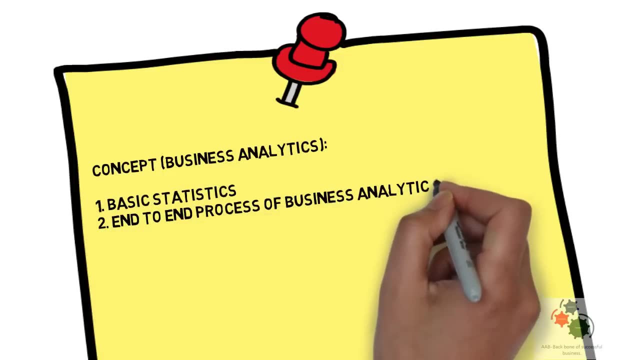 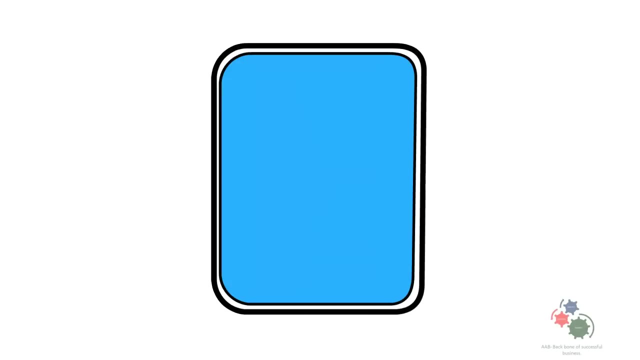 Please view this video till end. In these videos I'll explain below concepts: basic statistics which you must need to understand if you want to learn business analytics. End-to-end process of business analytics. mostly used Model Validation Concepts. Below are the statistical concepts which you must need to know to understand business analytics.